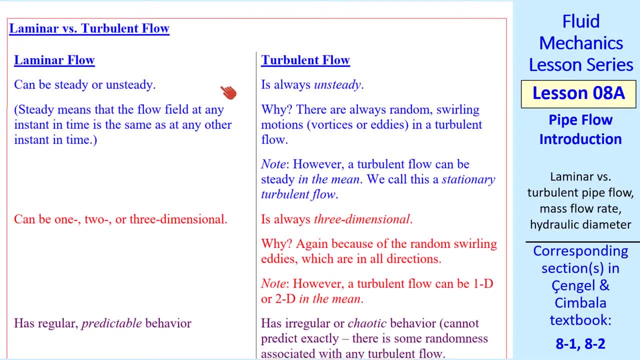 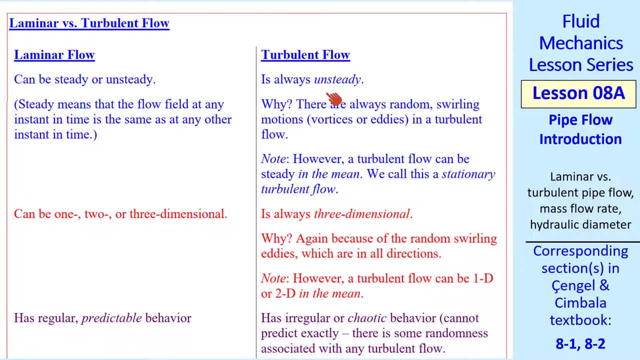 Now I want to briefly compare laminar versus turbulent flow. I have two columns with corresponding comments. Laminar flow can be steady or unsteady, but turbulent flow is always unsteady. With turbulent flow, there's all these eddies mixing things around. 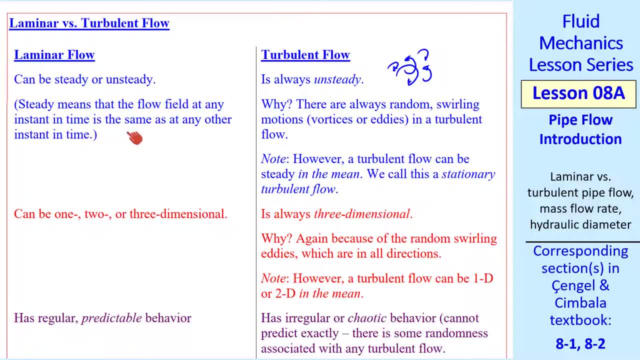 By the way, steady means that the flow field at any instant in time is the same as at any other instant in time, But because of these vortices or eddies in a turbulent flow it's always unsteady. However, turbulent flow can be steady in the mean. 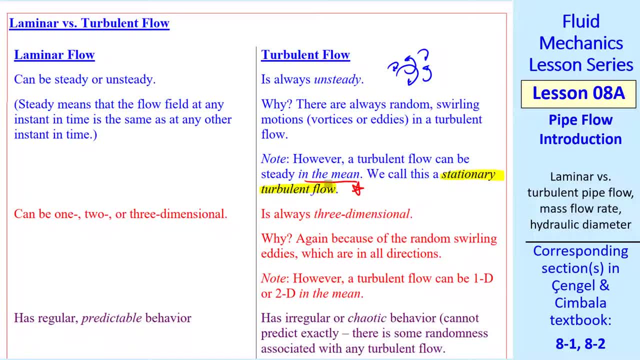 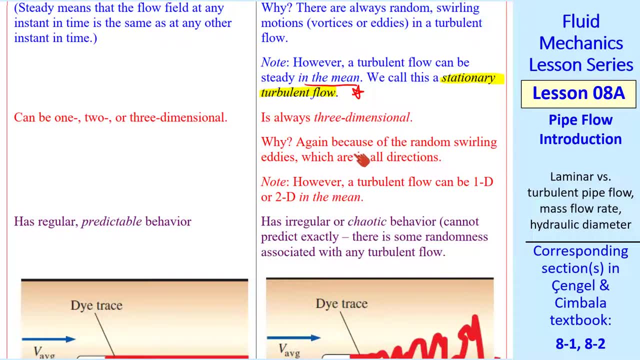 and that's what we'll generally look at in this course. We call that a stationary turbulent flow. Laminar flow can be one-, two- or three-dimensional. Turbulent flow is always three-dimensional, Again because of these random swirling eddies. 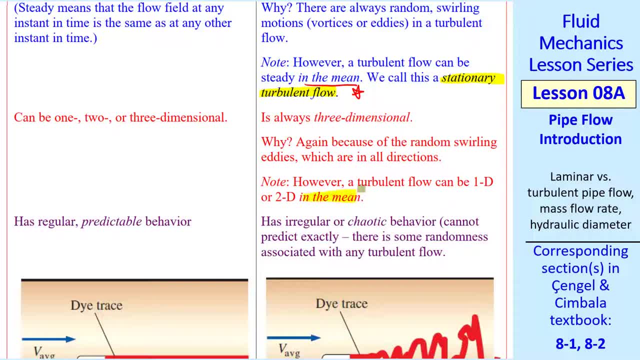 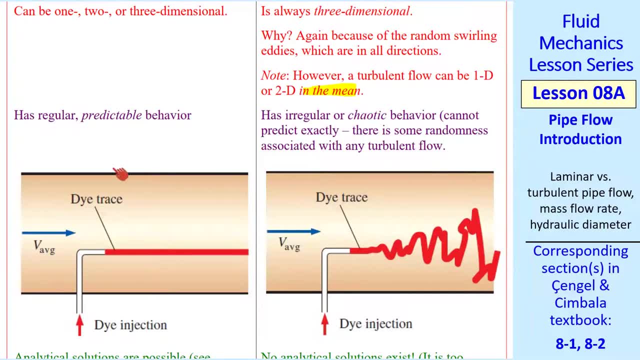 But a turbulent flow can be 1D or 2D in the mean- Again, that's what we'll always talk about in this course- Laminar flow has regular predictable behavior. For example, when you inject dye, you get a nice streak line, that's straight. 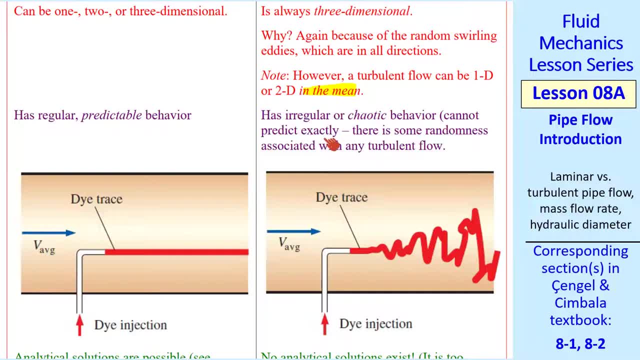 Turbulent flow has irregular or chaotic behavior which cannot be predicted. There's always randomness. If you inject dye into a turbulent pipe flow, you'll get all kind of random motion of the streak line. For laminar flow, analytical solutions are possible. 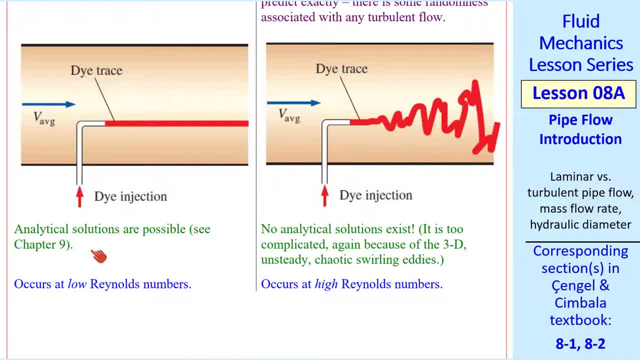 We do some of those in Chapter 9 of the Chang'e Symbolic textbook. For turbulent flow. no analytical solutions exist. It's too complicated because of the unsteady 3D chaotic eddies, So typically we solve for them. 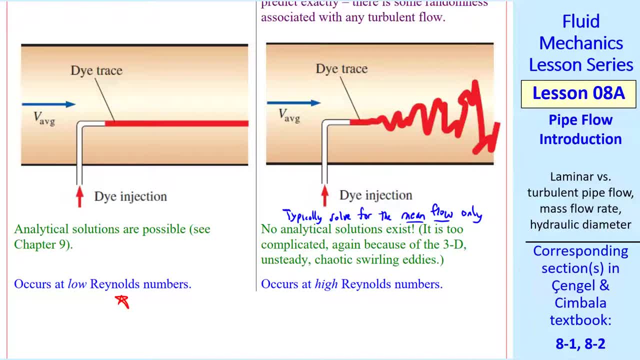 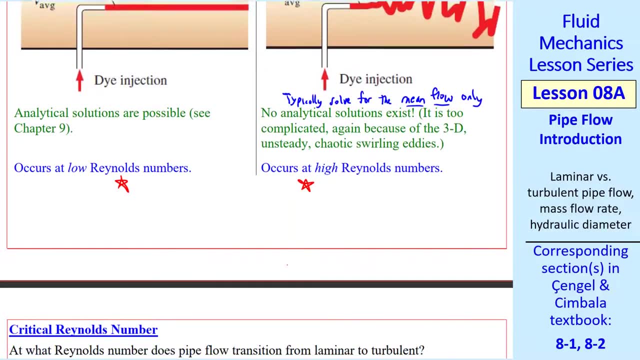 with the mean flow only. For the purposes of this course, it's important to know that laminar flow occurs at low Reynolds number and turbulent flow occurs at high Reynolds number. This leads to a discussion of critical Reynolds number, In other words, at what Reynolds number? 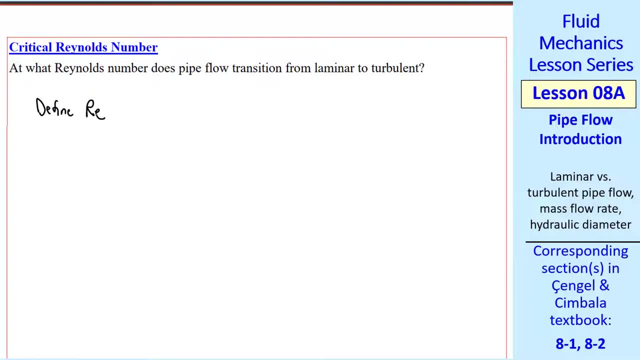 does pipe flow transition from laminar to turbulent? First let's define the Reynolds number For a given pipe flow. we have some average speed, v, pipe diameter, d and flow properties, mu and rho. Note that d is the inner diameter, of course. 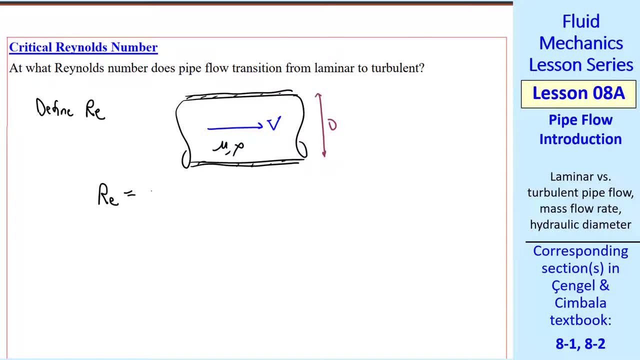 The outer diameter has nothing to do with the flow. We define our Reynolds number as rho, vd over mu, But recall from a previous lesson that nu is the viscosity over rho, which we call the kinematic viscosity. So a simpler expression for Reynolds number is vd over nu. 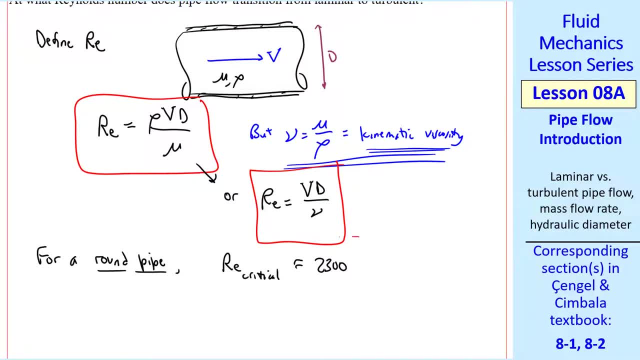 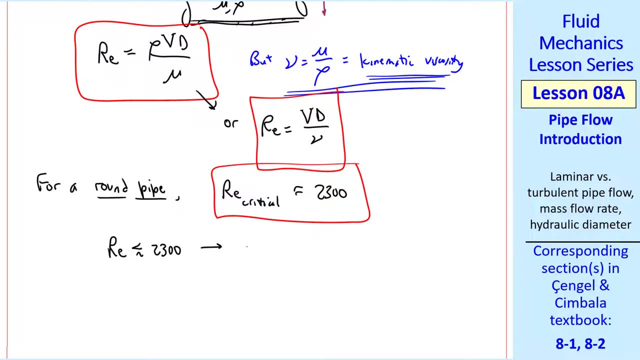 For a round pipe the critical Reynolds number is around 2300.. What that means? that for typical pipe flows, if Reynolds number is less than about 2300, we have laminar flow in the pipe If the Reynolds number is between 2300 and about 4000,. 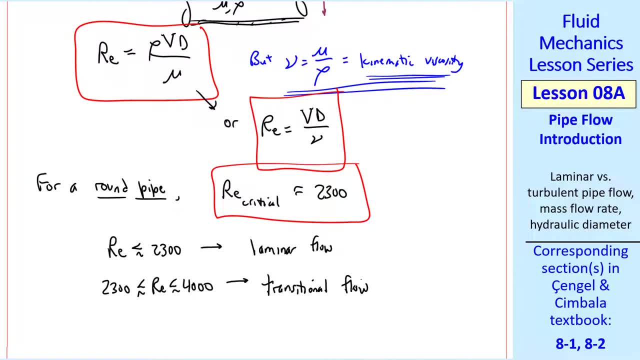 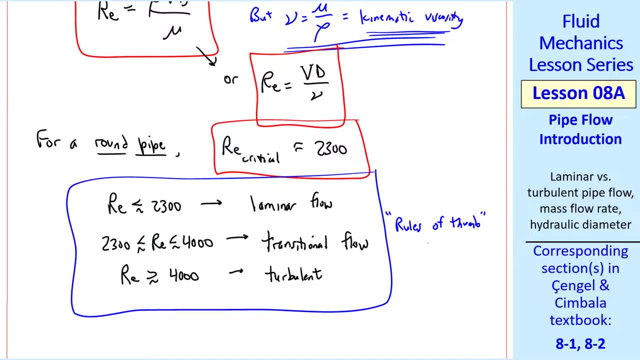 we have transitional flow which is kind of between laminar and turbulent, And if Re is greater than about 4000, the flow is turbulent. These are just so-called rules of thumb, meaning they're approximate values. You can have turbulent flow at Reynolds numbers. 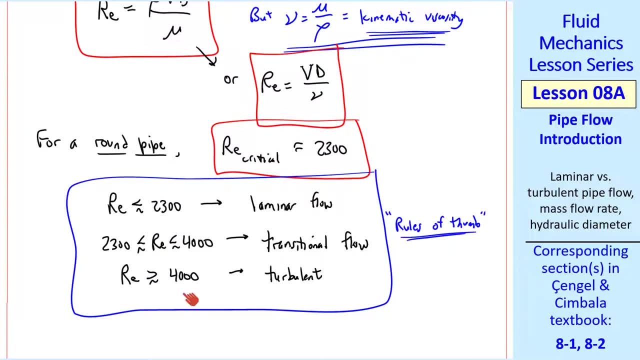 in this range and sometimes even below 2300, if your pipe is very rough or if you have lots of vibrations and stuff like that. Likewise, you can have laminar flow to Reynolds numbers above 4000 if you have very smooth pipe walls. 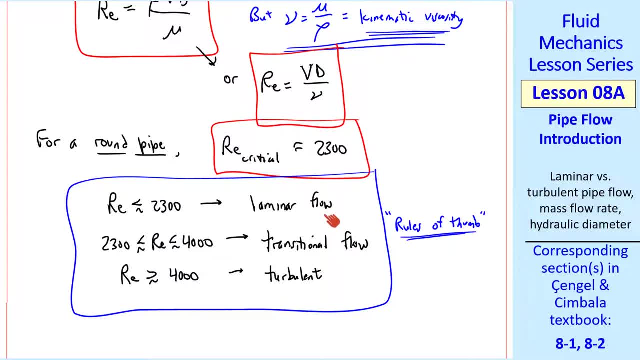 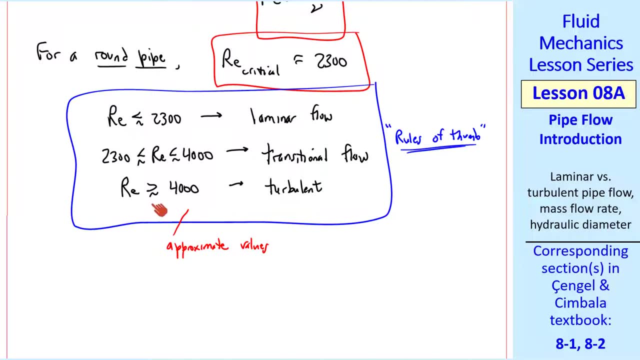 and very carefully controlled inlet and very low vibrations. In other words, these are just approximate values, But we'll use them to define whether the flow is laminar or turbulent or transitional. I'll make a list of how these values can change. They would vary with pipe roughness. 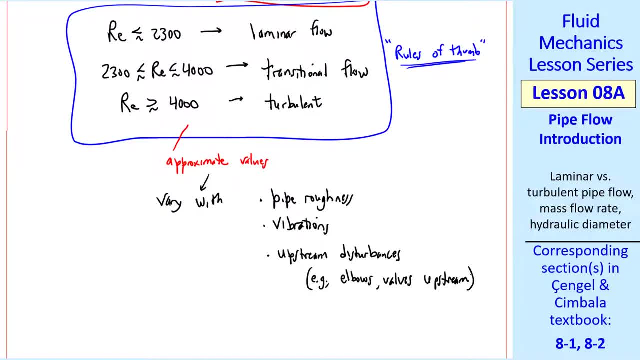 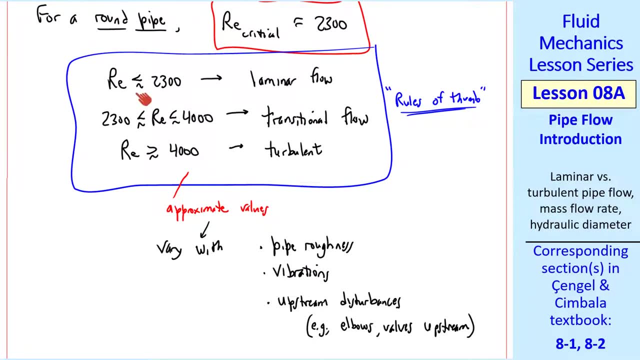 vibrations, upstream disturbances, for example elbows or valves in the flow upstream that disturb the flow and can cause it to be turbulent or transitional, even for Reynolds numbers in the laminar range. So keep in mind that these values are not set in concrete. 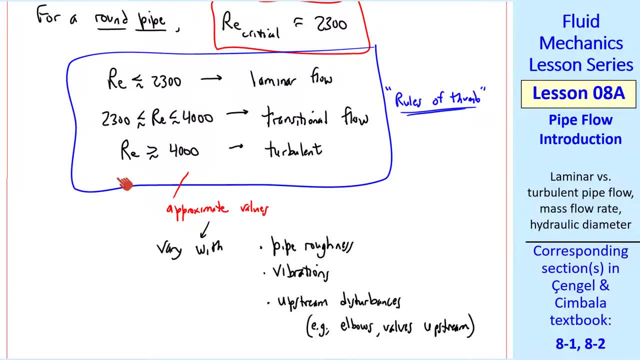 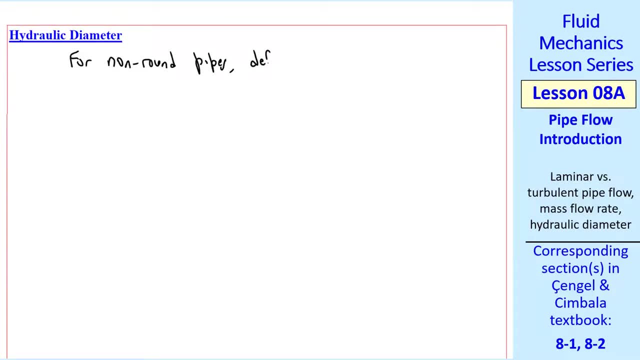 They vary, But we'll use these values to analyze our problems. Now I want to discuss hydraulic diameter. This is used for non-round pipes, for which we define the hydraulic diameter: d sub h is 4ac over p, where ac is the actual cross-sectional. 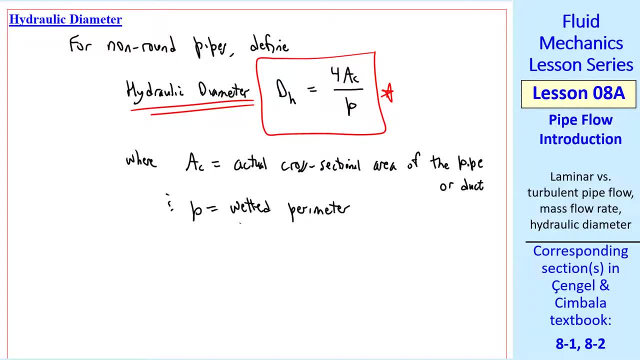 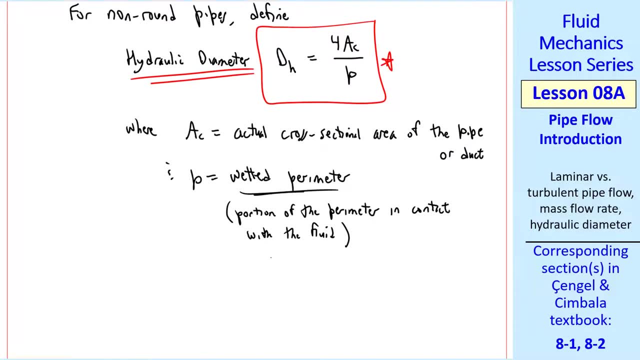 area of the pipe or duct And p is called the wetted perimeter, which is the portion of the perimeter in contact with the fluid. It's the actual perimeter if you're talking about a gas or a pipe that's totally filled with a liquid. 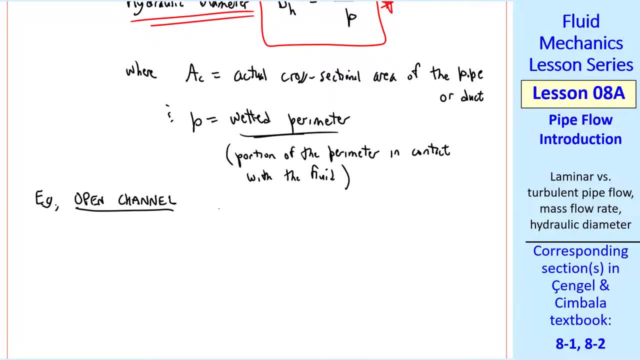 But we have to be careful if we have a channel. Let's take, for example, an open channel where water or some other liquid fills up only a portion of the channel. Suppose this height is 1 meter and its width is 2 meters. 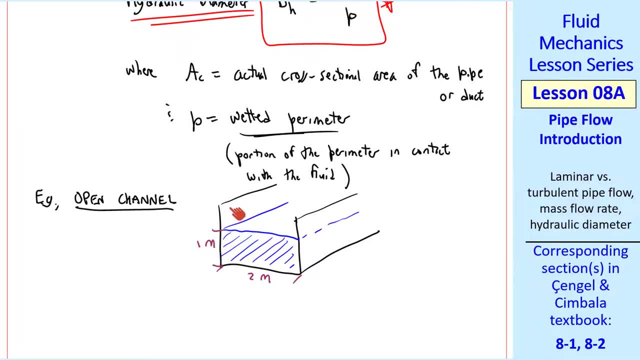 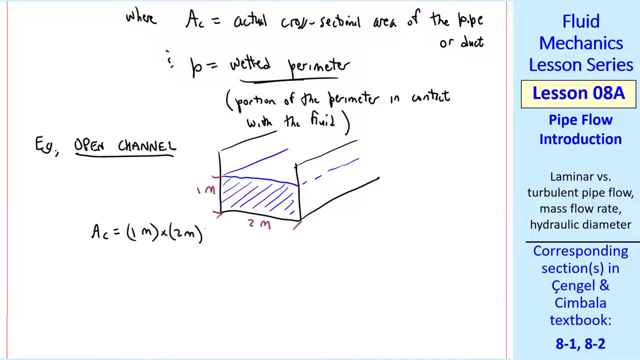 You don't count this portion of the inside of this channel because it's not exposed or wetted by the liquid. In this case, the cross-sectional area is 1 meter times 2 meter. This is that portion of the area that is filled by the liquid. 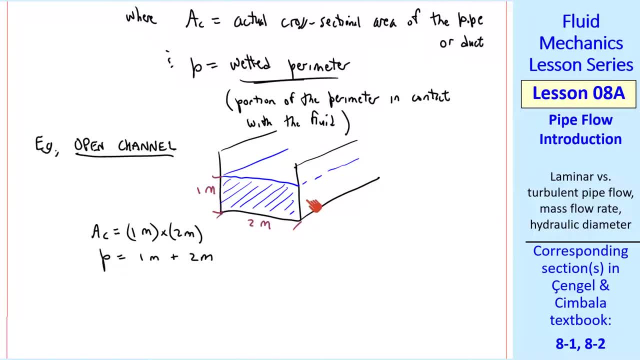 And p would be 1 meter plus 2 meter plus another meter here, which equals 4 meters. So dh would be 4ac over p, or 4 times 2 square meters over 4 meters. So the hydraulic diameter is 2 meters in this example. 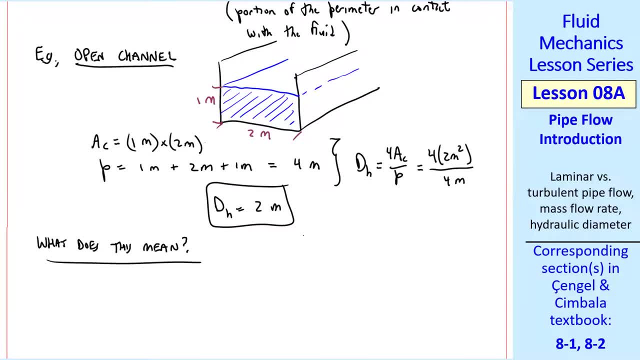 What does this mean and why do we use hydraulic diameter? As we'll see later, there are correlations and empirical equations for Darcy friction factor F as a function of Reynolds number, And those are all based on round pipes. We'd like to use these correlations. 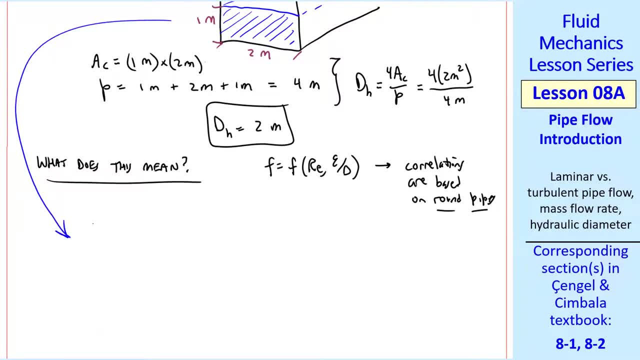 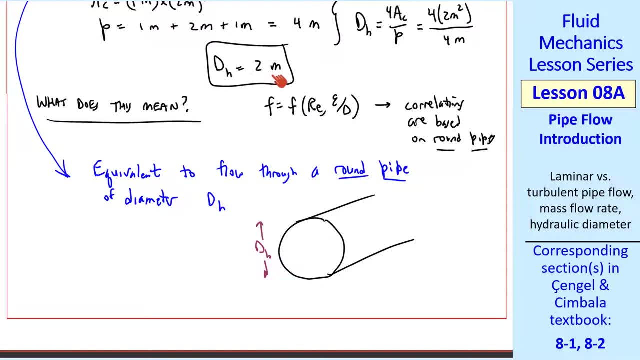 even if the pipe is not round. So what we're saying is that this actual channel is equivalent to flow through a round pipe of diameter dh. Here we calculated our dh as 2 meters, So flow through this circular pipe is equivalent to flow through this. 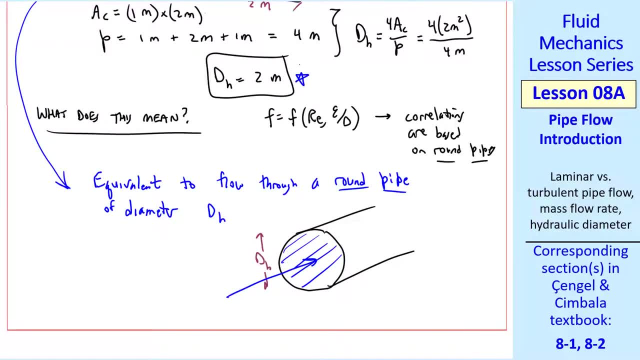 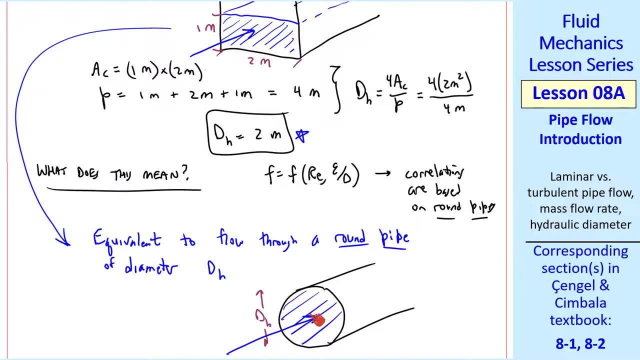 actual pipe or channel if we use hydraulic diameter. But there's a problem with doing this, namely that this cross-sectional area is not the same as this cross-sectional area. So when calculating m dot or v dot, use the real cross-sectional area ac. 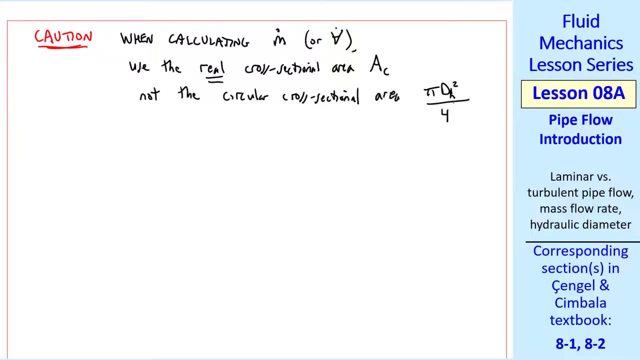 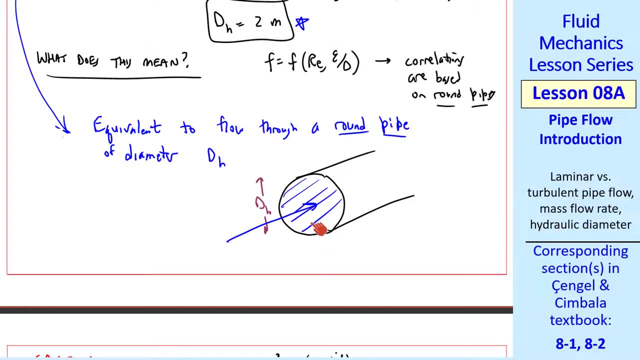 not the circular cross-sectional area, which would be pi dh squared over 4.. In other words, this area. We must use this actual area, not this area when calculating m dot or v dot. Mathematically, when we use m dot equal rho va. 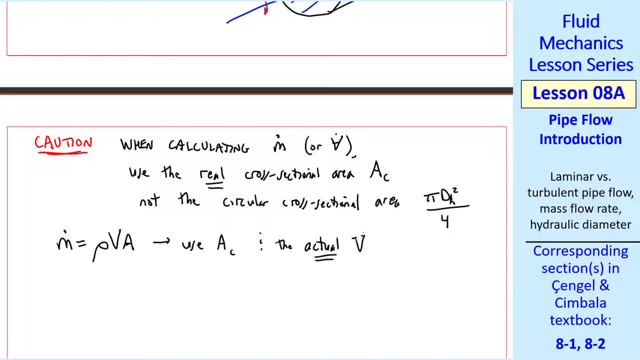 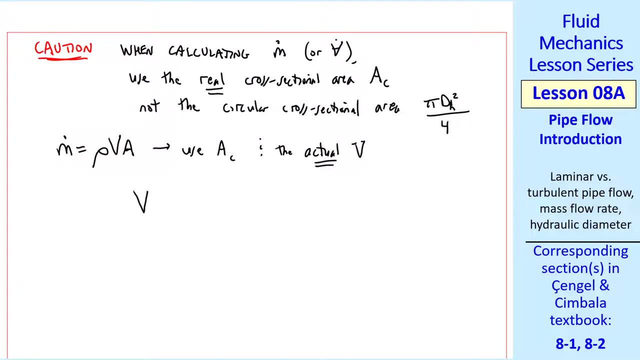 we use ac, the actual cross-sectional area, and the actual v, which is the actual average speed through the non-circular pipe. So when you have a non-circular pipe and you know mass flow rate, you calculate v as m dot over rho ac. 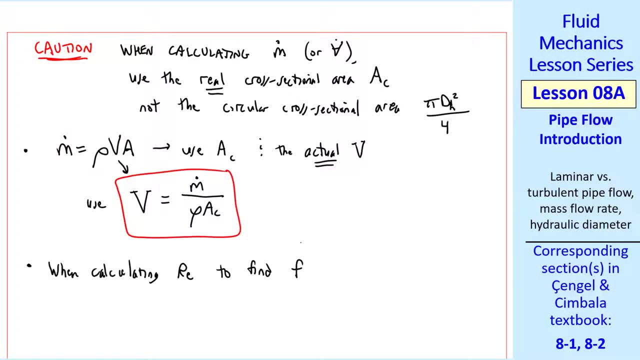 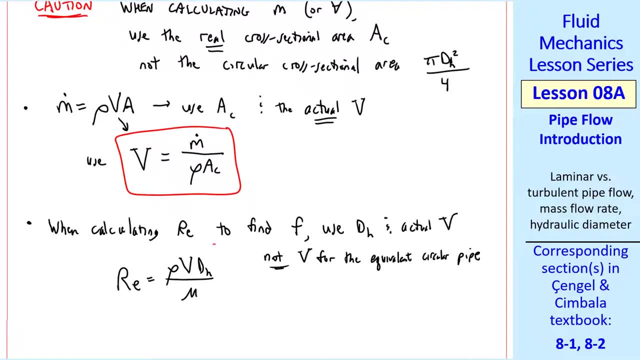 But when you're calculating Reynolds number to find Darcy friction factor, for example, we use dh and the actual v, not v. for the equivalent circular pipe, Re is rho v, dh over mu. For our above example, suppose the volume flow rate. 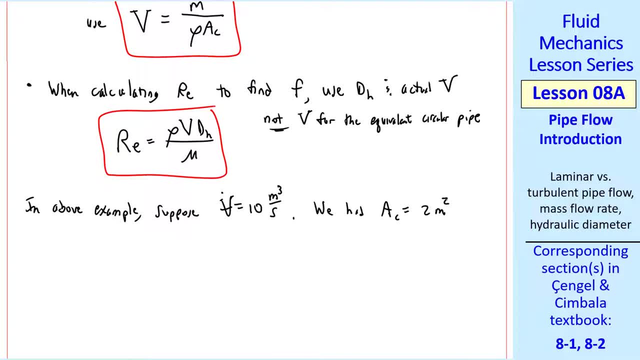 is 10 meter cubed per second. We had calculated that the actual cross-sectional area was 2 meters squared, so the average speed is v dot over ac or 5 meters per second. Use this value in calculating Reynolds number, The equivalent round pipe. 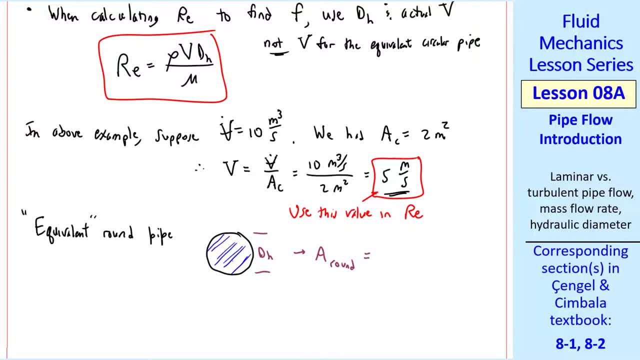 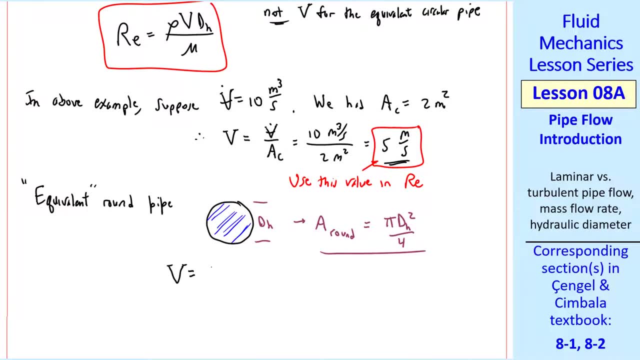 has a hydraulic diameter dh, so the cross-sectional area a round is pi dh squared over 4.. If we would use that to calculate the average speed, we would get v dot over pi dh squared over 4, which turns out to be 3.183 meters per second. 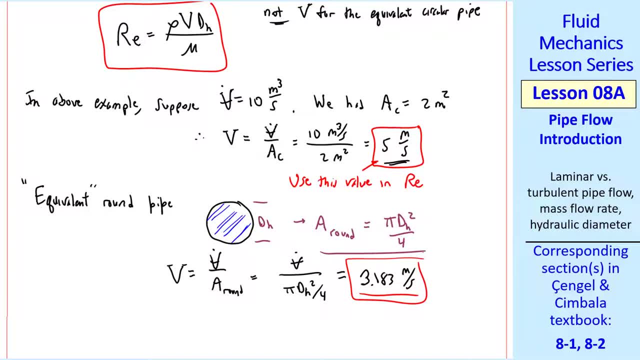 You might be tempted to use that v to calculate your Reynolds number, since we're kind of pretending that we have this round pipe. but we have to be careful to use this speed, not this speed. Do not use this speed in calculating the Reynolds number. 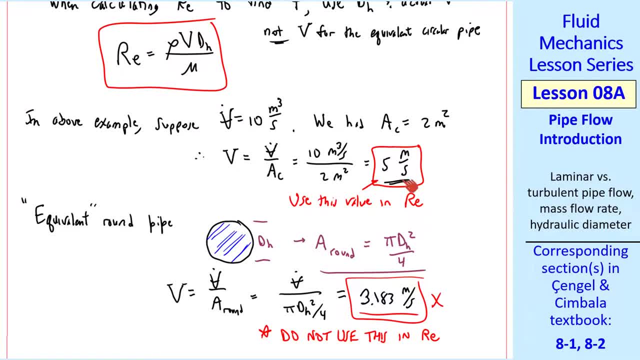 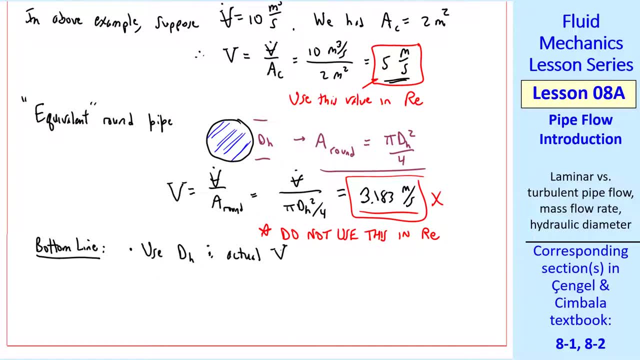 Once you know the actual average speed, in this case 5 meters per second, and we know dh, we can calculate a Reynolds number. So the bottom line: use dh and the actual average speed to calculate Reynolds number. then use that Reynolds number. 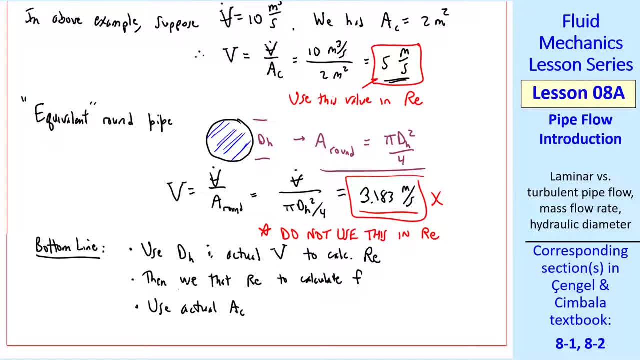 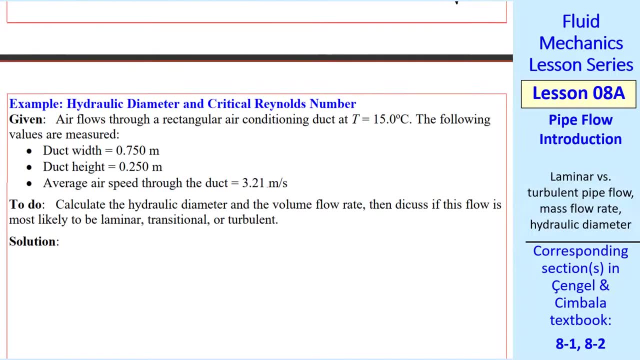 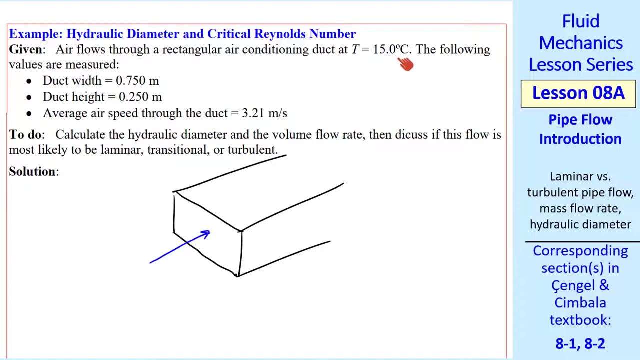 to calculate Darcy friction factor and use the actual cross-sectional area and the actual average speed for calculation of m dot or v dot. Let's do an example. Suppose we have a rectangular air conditioning duct. Air flows through at a cool 15 degrees C. 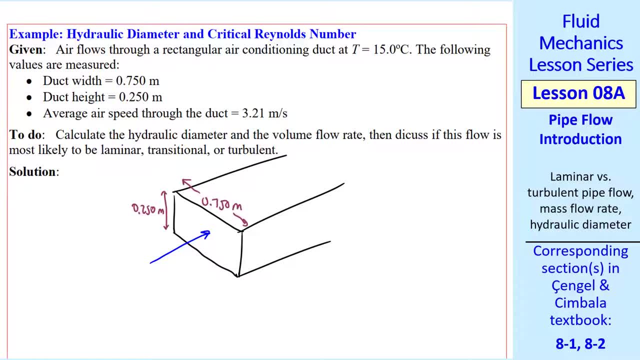 and we're given the duct width and the duct height, as well as the actual average speed through the duct. We want to calculate the hydraulic diameter volume, flow rate and then try to determine if this is laminar, transitional or turbulent. 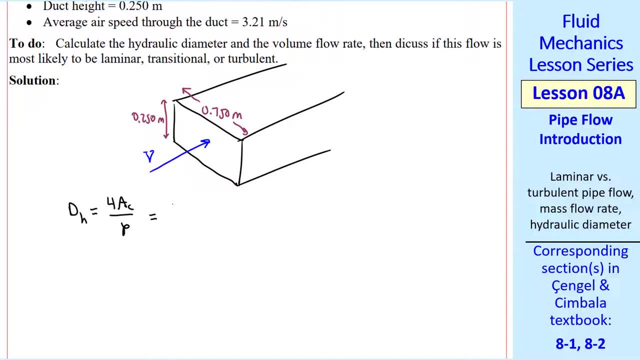 Let's use our equation for hydraulic diameter, For AC over P, the cross-sectional area is the width times the height, which is that cross-sectional area And the perimeter includes this height, this width, this height and this width, since the air wets, the whole surface.